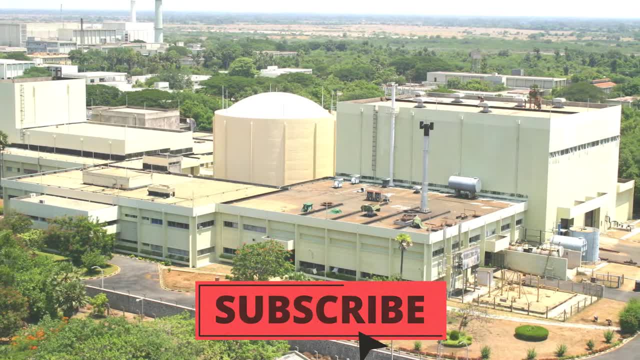 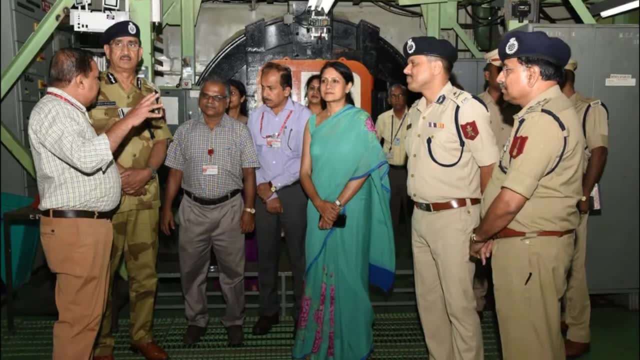 until the end of the year. launch of the PFBR, which is the flagship of India's FAST program. The fundamental decision to start work on the RAPID program was made in India in 1968.. A year later, the nuclear departments of India and France entered into an agreement. 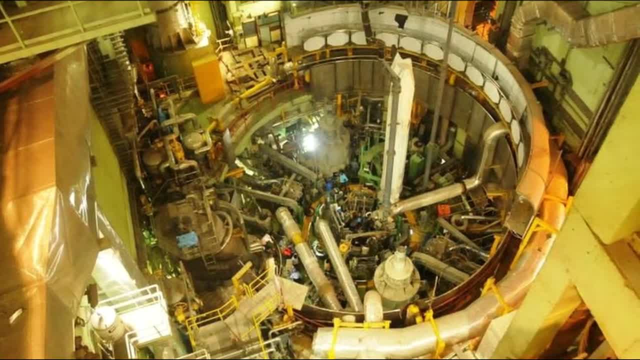 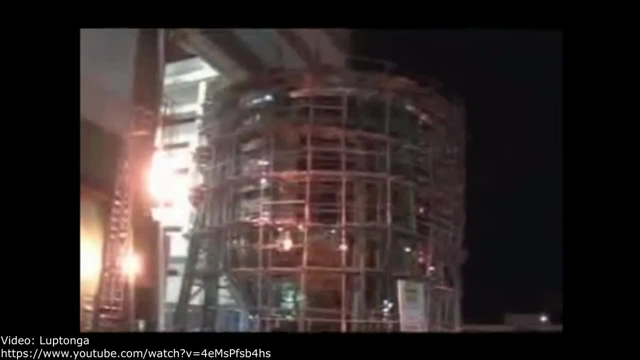 on cooperation in the construction of a FAST research reactor. In 1971, a nuclear center was established at Kalpakkam and in 1972, construction of the FBTR started. Around 1978, it was decided to refocus. the FBTR on carbide fuel. On October 18, 1985, the reactor reached criticality for the first time, and on March 7, 2022, it was brought to its design capacity of 40 thermal megawatts. 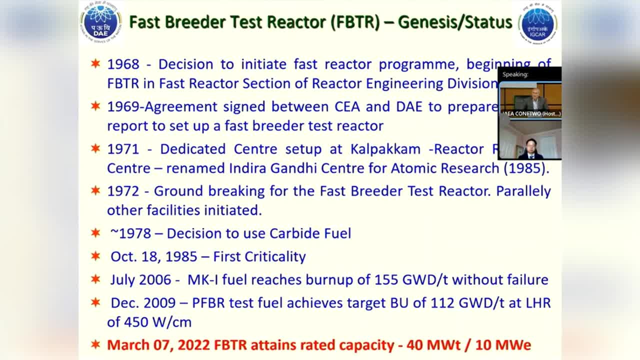 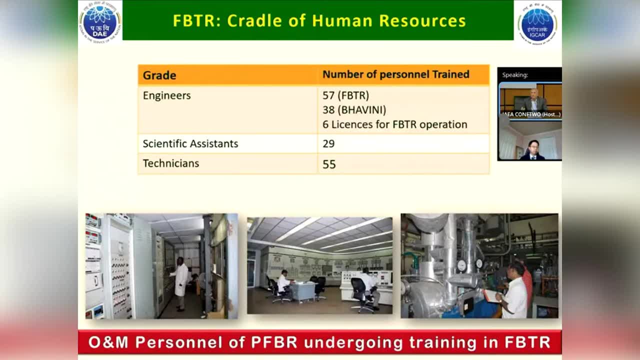 or 10 electrical megawatts. for the first time Throughout its history, FBTR has become a forge of resources for the nuclear industry. More than 100 engineers and more than 50 technicians, as well as almost 30 scientists, have been trained at the reactor. Various types of fuel, the FBTR's 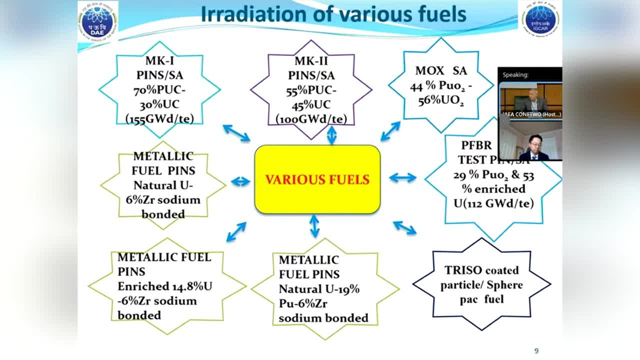 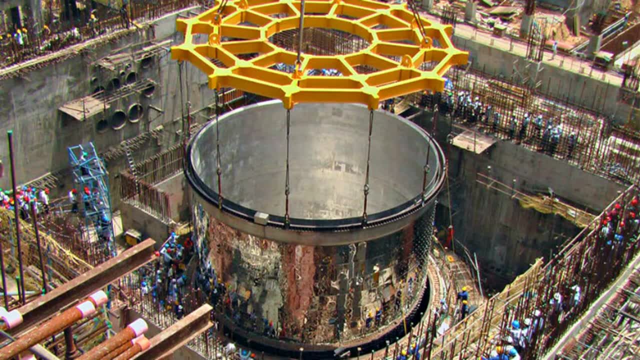 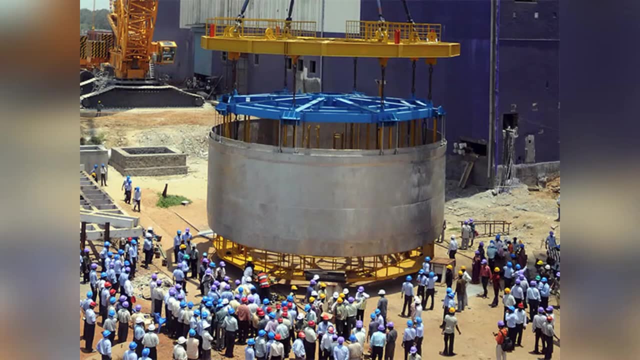 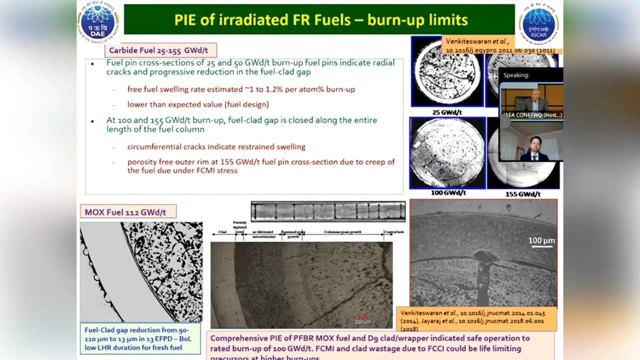 types of fuels were tested at the reactor: carbide, metal oxide and even triso. in addition, irradiation experiments were carried out with various structural materials. the speaker recalled that the fbtr reactor had successfully demonstrated the closure of the fuel cycle, thanks to a pilot plant for the reprocessing of irradiated fuel commissioned in 2003.. to date, the fbtr reactor 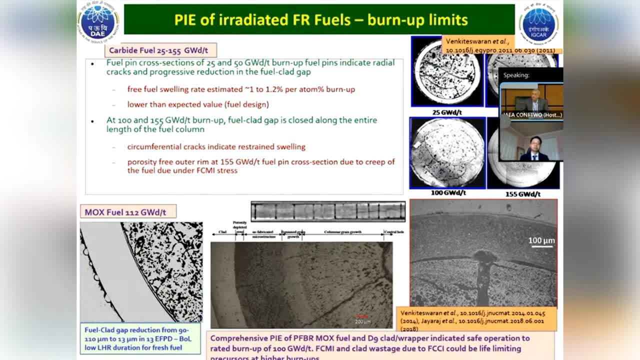 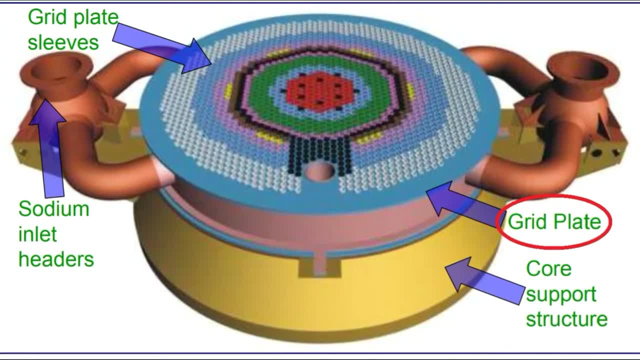 has worked for 36 years and the question arose of its extension. it is quite realistic, given that the reactor reached its design capacity just recently. to reduce the dose load on the bottom plate of the reactor, which is the most vulnerable component, it was decided to modify the design of 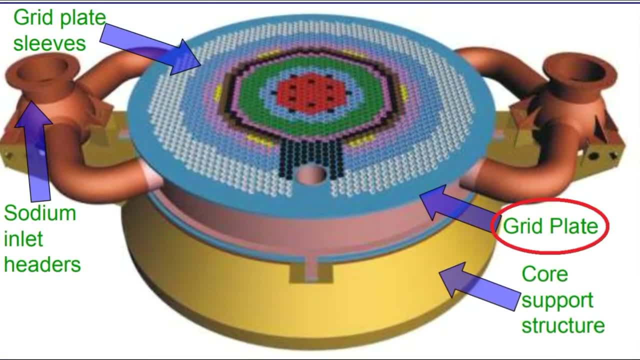 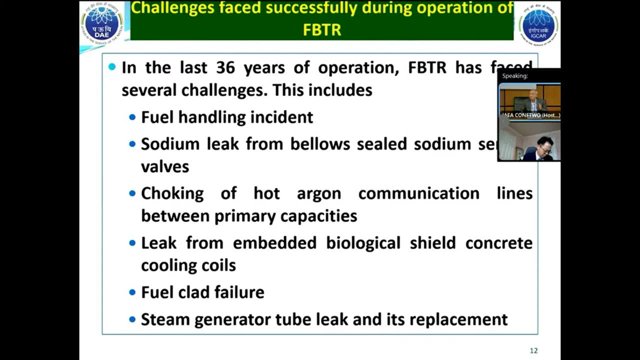 the fuel assemblies and add tungsten carbide pellets to it as a bottom shield. largely due to this measure, it should be possible to leave the fbtr in service until 2034-2035. of course, the part devoted to india's plans to develop a rapid program and close the nuclear fuel cycle is of 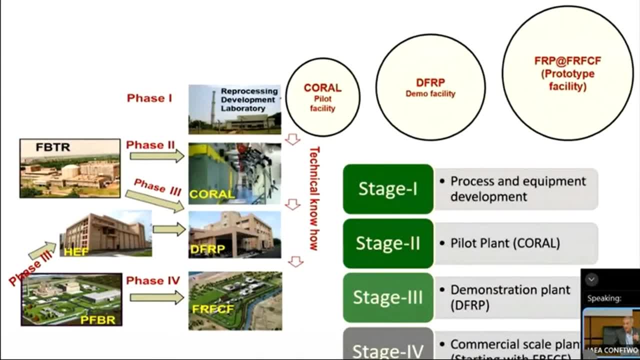 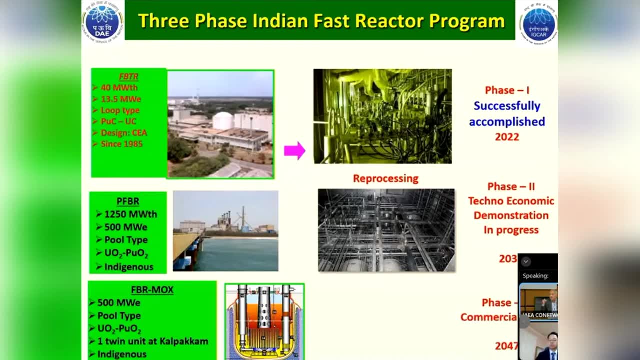 greatest interest in the report. the speaker announced that in 2022, india has successfully completed the first phase of the fast program, which included the operation of the fbtr reactor and the closing of its fuel cycle. the second stage, called a feasibility study by the speaker, should